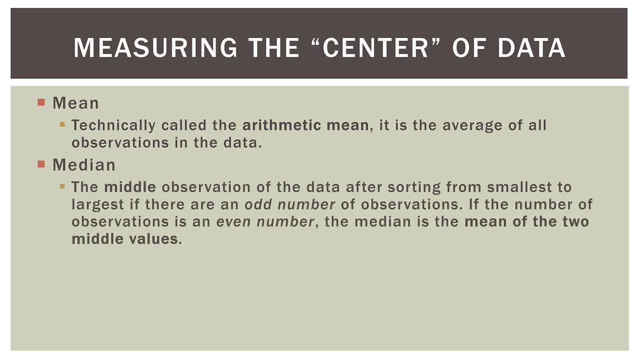 to you probably. The next is the median, And for students just starting in stats, this can be a new concept. But basically the median is the middle observation of a data set. So what we do is we sort them from smallest to largest. 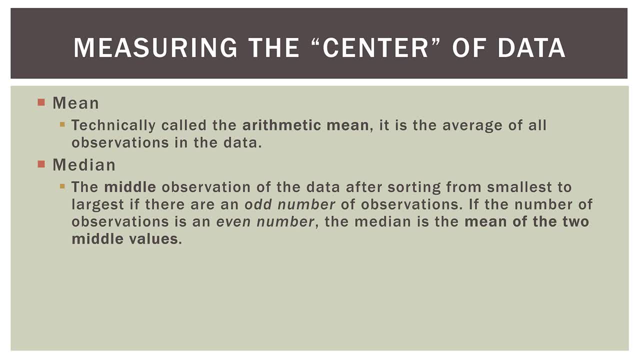 And if there are an odd number of observations, it's the one literally in the middle after sorting. If the number of observations is an even number, the median is the mean or the average of the two numbers in the middle. 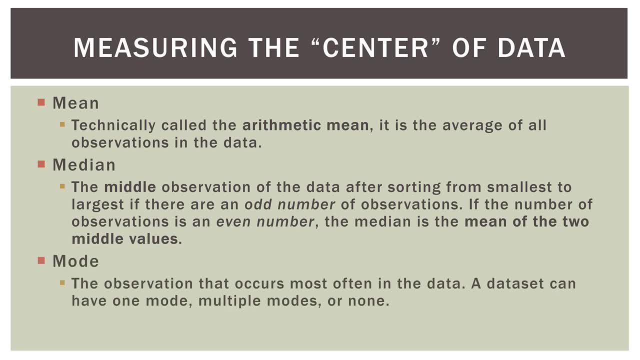 And we'll see that in a couple minutes. The mode is simply the observation that occurs most often in the data, or the most frequently occurring observation. Now, a data set can have one mode, it can have multiple modes or it could have no mode at all. 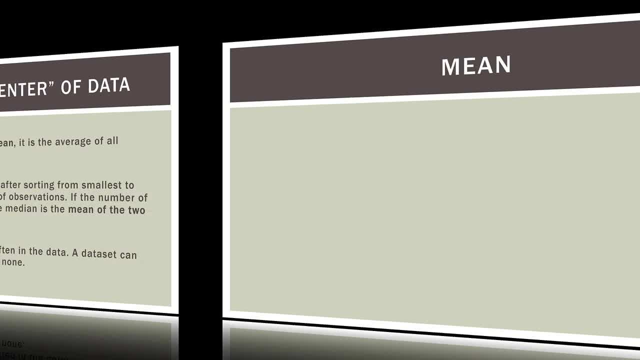 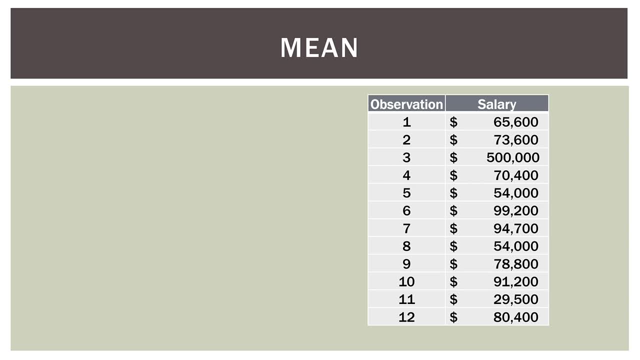 It simply depends on the data you have. So first the mean. So here are some salary data I created. So we have 12 observations and 12 salaries. So to calculate the mean, it's very simple: We add or sum up all the observations. 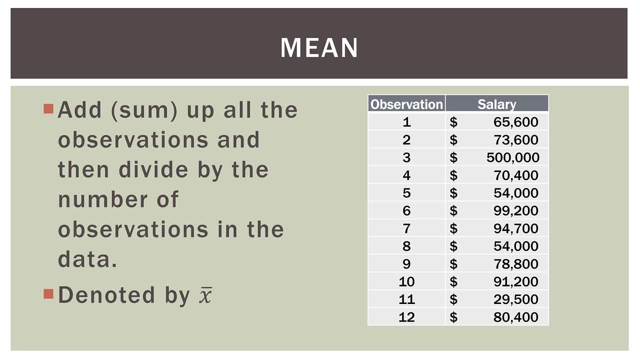 and then divide by the number of observations in the data. So in this case we would add up all the salaries and then we would divide by 12.. And in notation we denote that by what's called x-bar. So it's an x with a bar over the top. 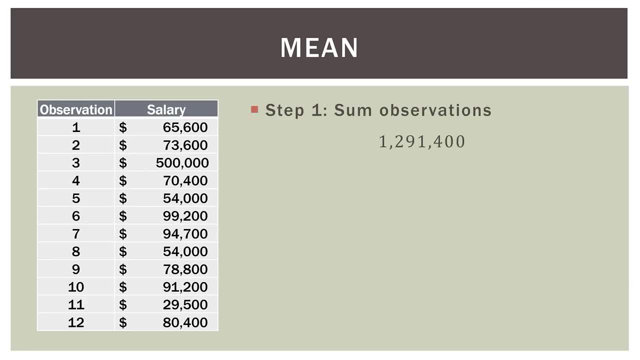 So step one. So step two. Step one: we sum our observations. When we sum all of our salary data, we have $1,291,400.. Step two: we count our observations. Now notice, I have the word length in parentheses there. 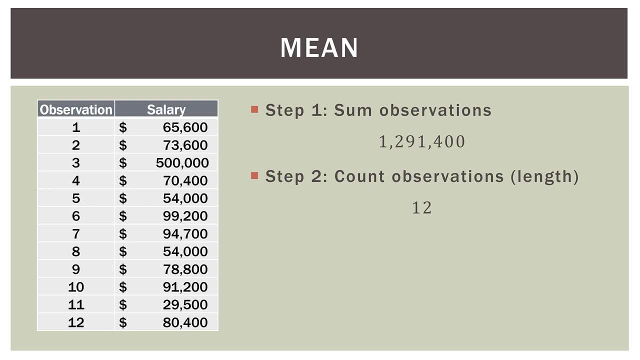 The reason I have length is because length is often how we describe a data set when we're doing programming applications. So in programming, when we have a data set like this, it's basically what's called an array. So the salary data here is an array with a length of 12.. 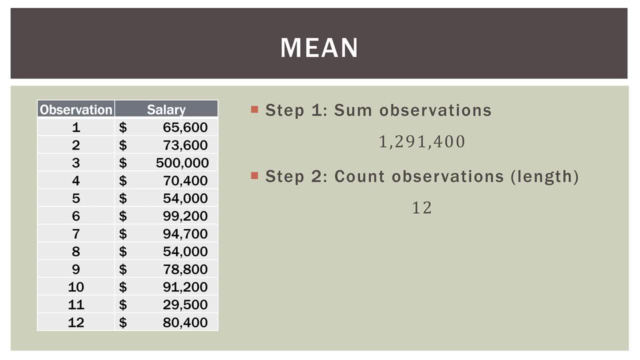 So, as students get more into coding environments, I like to describe things in ways that you're gonna see in code. But if you're not into that or not going into that, it's simply the count of the number of observations. So in step three we just divide the sum by the count. 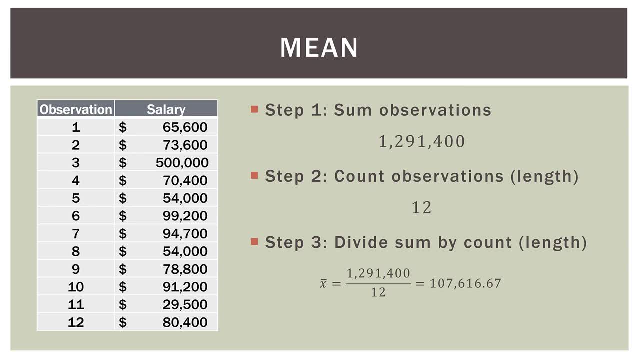 or the length of our data set. So we have $1,291,400 divided by our 12 observations and we end up with a sample mean of 107,000.. $107,616.67.. So that is the mean or the average salary. 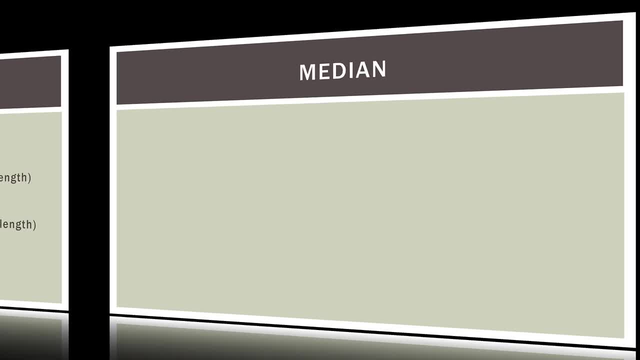 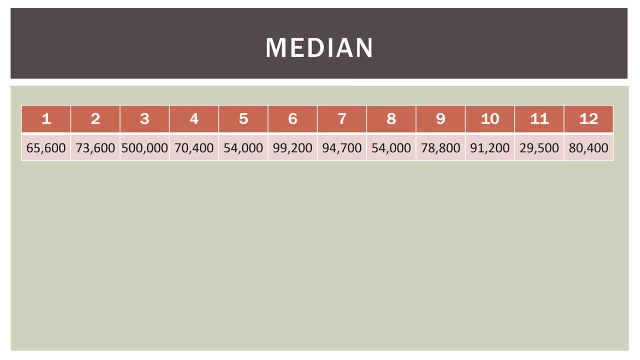 of our 12 observations. So next we have the median. So here is our data, same numbers, but I put it in a horizontal format and you'll see why here in a second. So observation one is 65,600, and so on and so forth. 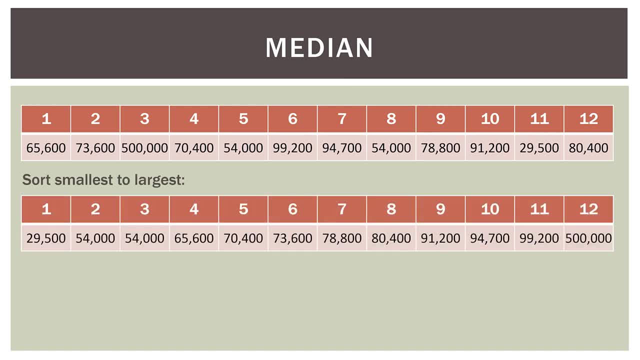 So to find the median, first, we sort our data from smallest to largest. So we can see here that we have a small salary of $29,500, all the way up to the maximum salary of $500,000.. So they are all in order from smallest to largest. 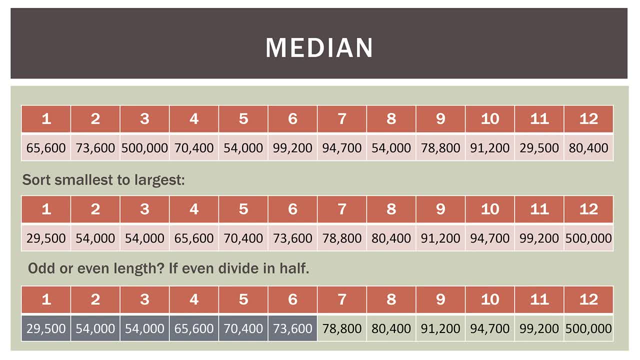 Next, we ask ourself: is our data odd or even length, or an odd or even count of observations? If it is, even as it is in this case, we then just divide it in half. So you can see, here I have the first six observations shaded. 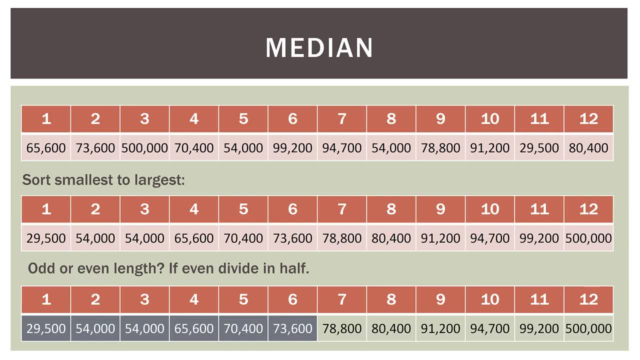 in a gray, and then I have the last six observations shaded in sort of a light brown, And because this data is an even number of count or an even length, we just divide it in half: Six on one side, six on the other. 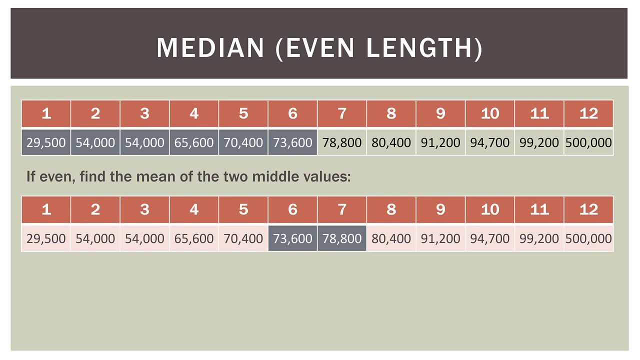 So here's where we left off. Now, since it's even, we find, the mean of the two middle values. So we can see here that observation six and observation seven, those are the two middle values on each side of that dividing line. so all we do 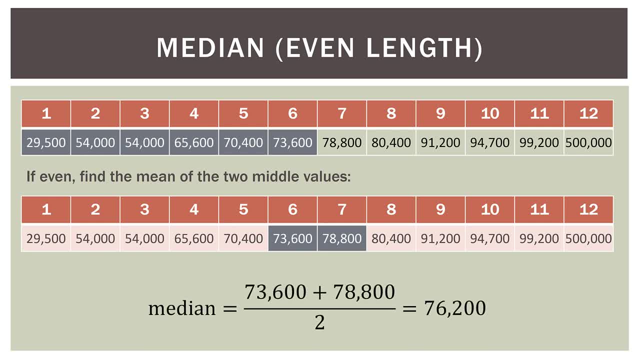 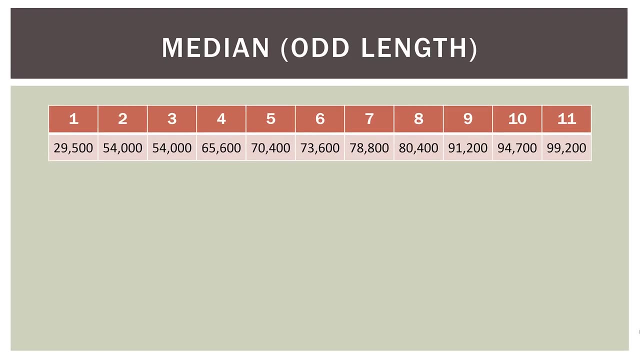 is find the average or the mean of those two values. So we have 73,600 plus 78,800, and then we just divide that by two. So our median in this case is $76,200.. So what if our data set has an odd number of observations? 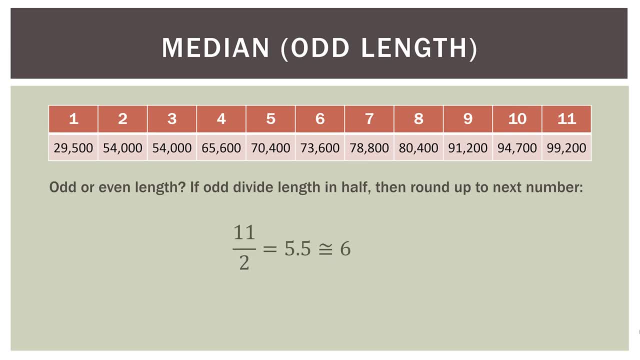 or is an odd length. Well, in this case we just simply divide our length or our count of observations in half and then round up to the next number. So in this case we have 11 observations. we divide that in half so we get 5.5,. 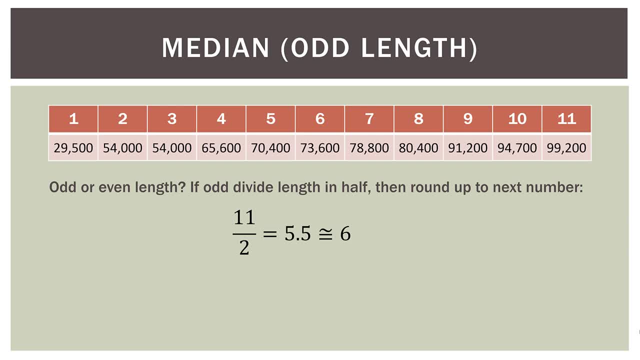 and then we just go ahead and round up to six, And it's the sixth value. that is our median. So in this case it's 73,600.. And if you notice that on either side of the sixth value we have five below it and five above it. 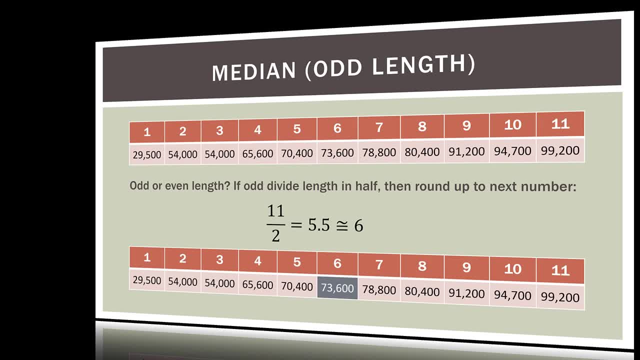 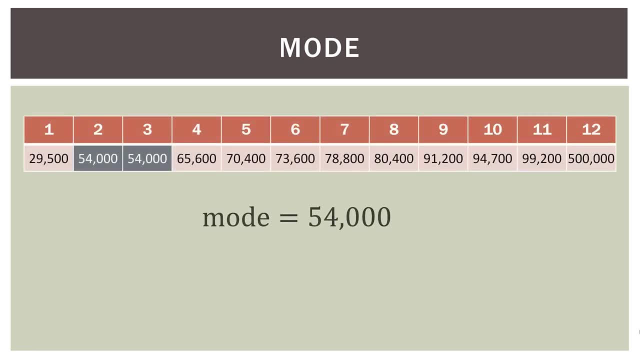 and the six is situated right in the middle. Now mode is very straightforward: It is the observation that occurs the most. So in this case we have two salaries of $54,000, and quite simply it's $5,000. 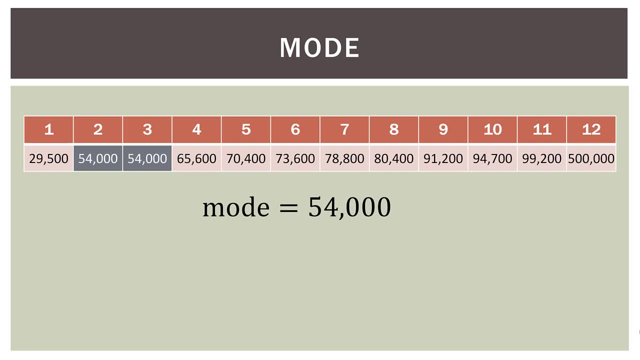 Simply, that is the mode. Now again, data sets can have more than one mode. So if we had two salaries that were $78,800, we would have two modes. We'd have a $54,000 mode and a $78,800 mode. 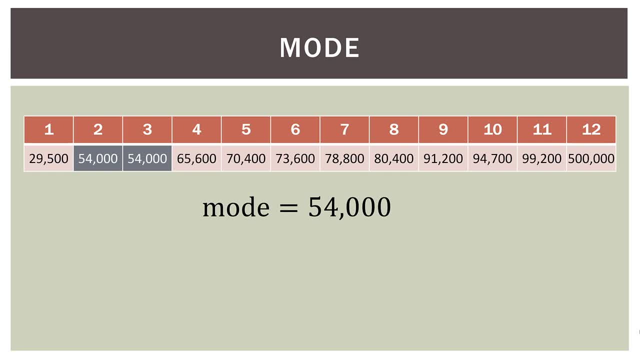 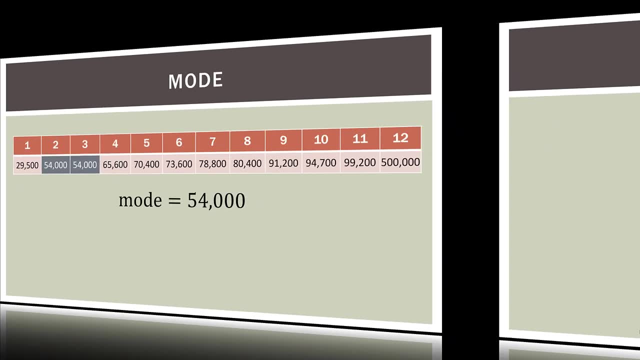 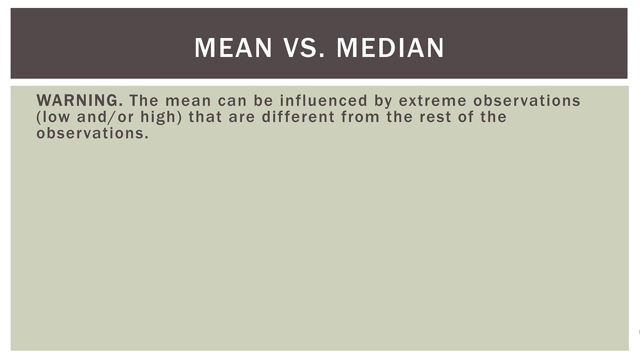 And some data sets don't have a mode at all. If all the values in our data set are unique, then none of them has more than one observation and therefore there is no mode, And this is actually a warning: The mean can be influenced by extreme observations. 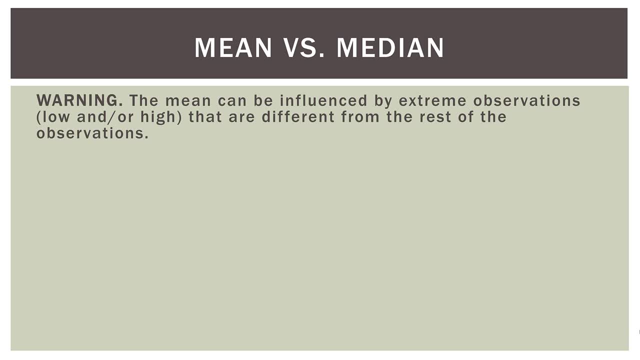 either low and or high that are different from the rest of the observations. So here's our data set from before. Notice we have someone in our data set that has a salary of $500,000.. Now look at the other 11 observations. 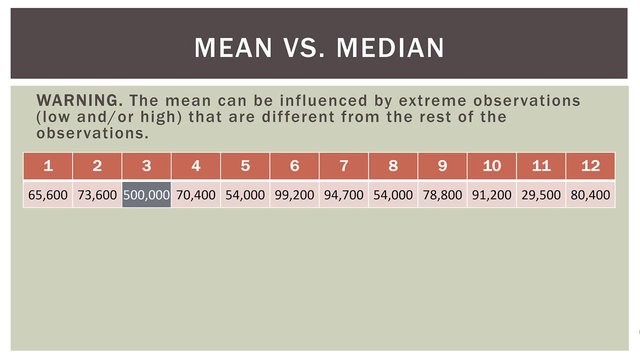 They all tend to be around like $75,000, give or take. So our sample data set, our sample mean, was $107,616.67.. However, our median was $76,200.. That is a massive difference, a huge difference. 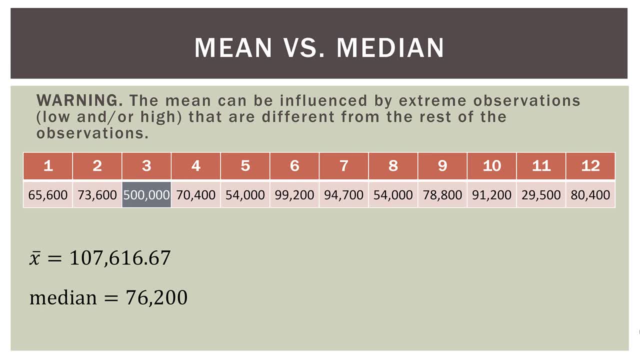 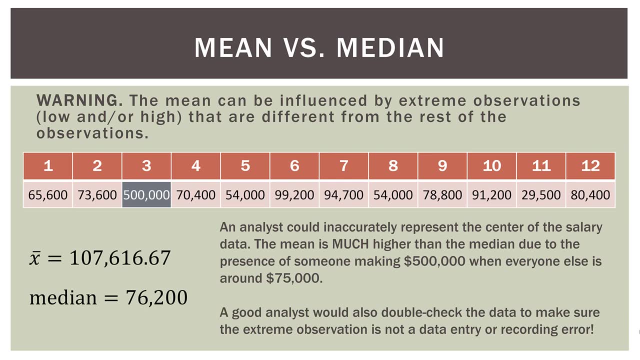 And the question is: which measure is more accurately representing the center of our data set? So an analyst could inaccurately represent the center of the salary data. This mean over here is much higher. This mean over here is much higher than the median due to the presence of someone making $500,000. 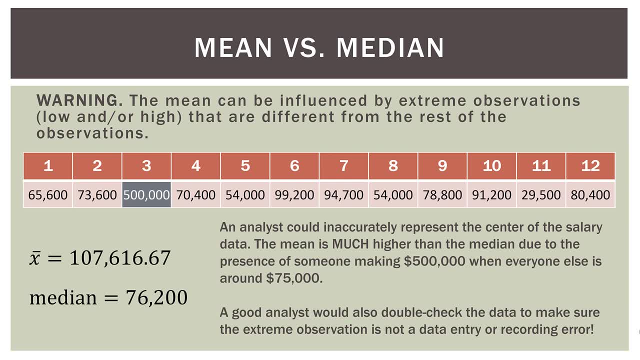 when everyone else is around $75,000.. Now also, a good analyst would double check that value. They would double check the data to make sure that extreme observation of $500,000 is not a data entry or recording error. In this case, it could be really, really easy. to type in $500,000 when it's supposed to be $500,000.. to type in $500,000 when it's supposed to be $500,000.. to type in $500,000 when it's supposed to be $500,000.. 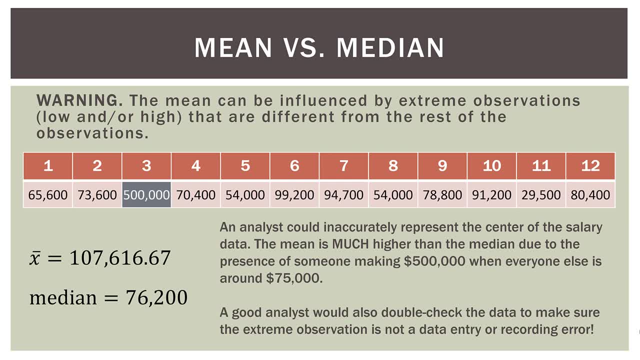 when it's supposed to be $500,000.. So if you do have an extreme observation in your data, don't just say to yourself: oh, that's just how it is. No, go back, look at your data, look at the records you have. 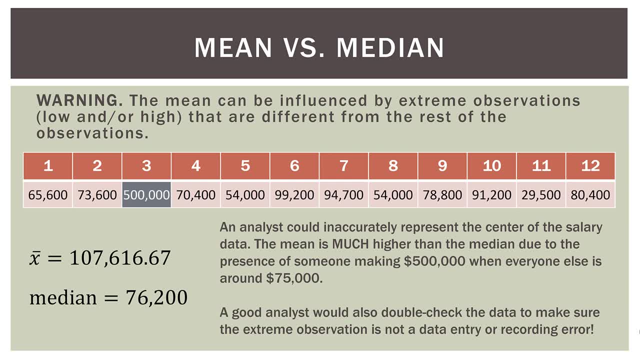 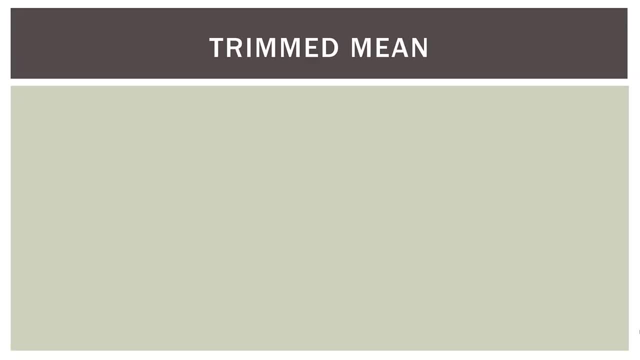 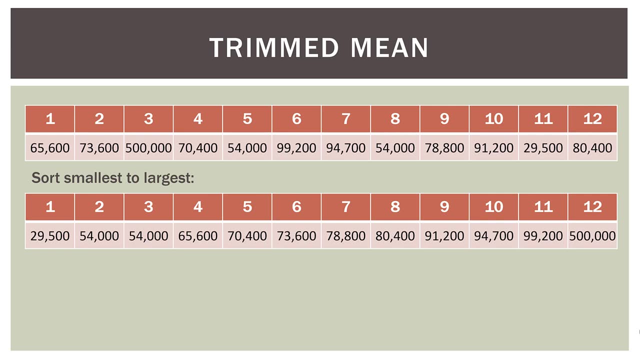 look at everything you have at your disposal to make sure that data is valid in the first place before beginning with your analysis. So our final concept is called the trimmed mean. So here's our data set again. Then what we do is we sort them smallest to largest. 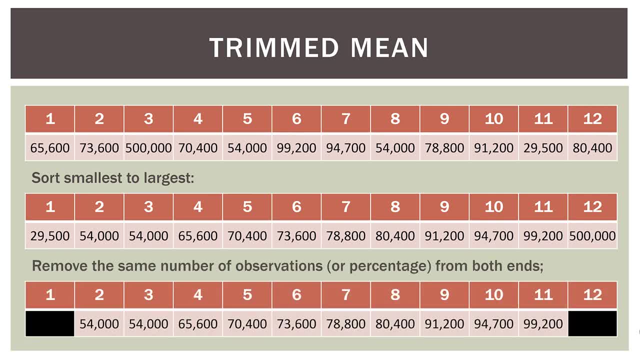 like we did with the median, and then we remove the same number of observations from each end of our data set. Now, sometimes this is expressed as a percentage, like a 5% trimmed mean or a 10% trimmed mean. Now, in the end it doesn't really matter. 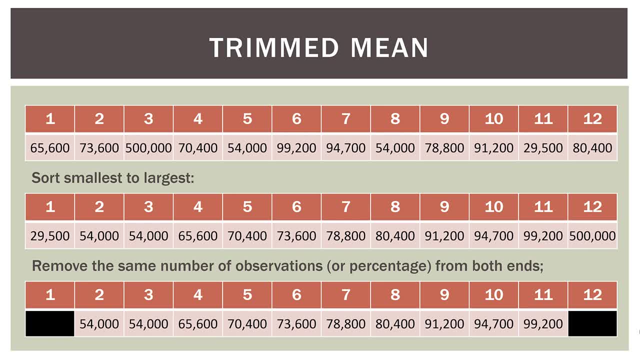 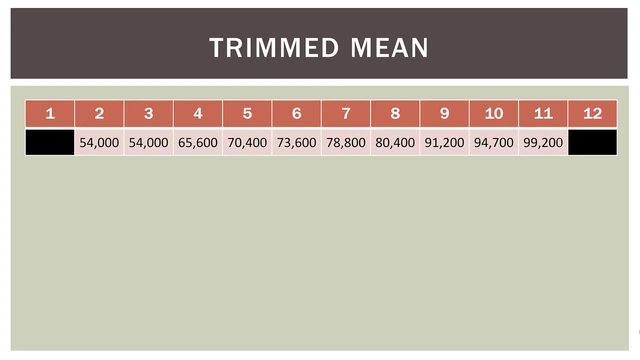 so long as you are removing the same number of observations from each end of the data set. So in this case we will remove the smallest of $29,500, and we will remove the largest of $500,000.. So from there we just calculate the mean again. 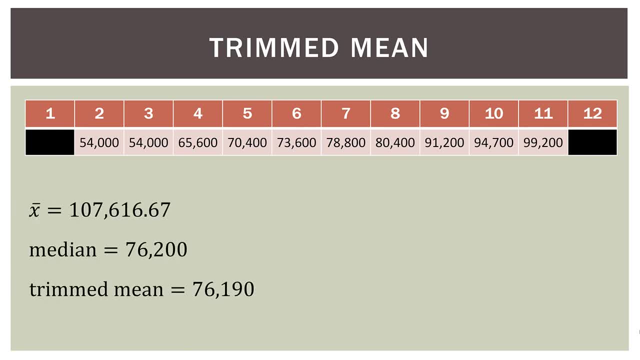 So in this case we have a sample mean, our original sample mean, of $107,616.67.. Our median was $76,200. And in this case our trimmed mean is $76,190.. Now look how close the median and the trimmed mean are. 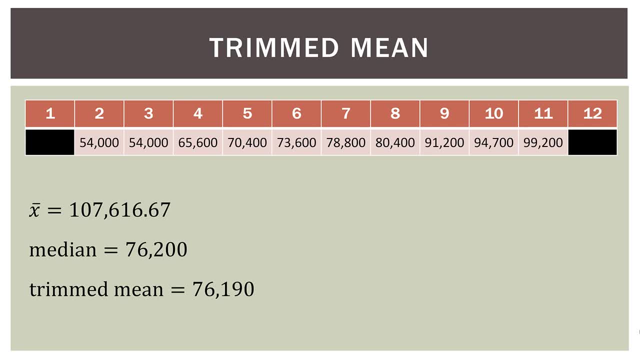 They're almost identical. So by removing the same number of extreme values on both ends, in this case, we got a value where the trimmed mean and the median are almost identical. So what we can do is conclude that that's probably the best representation of the center of our data. 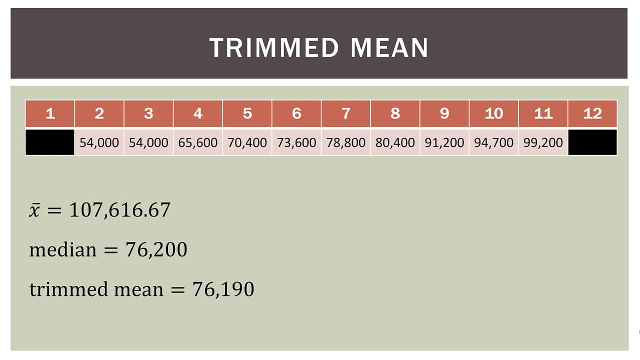 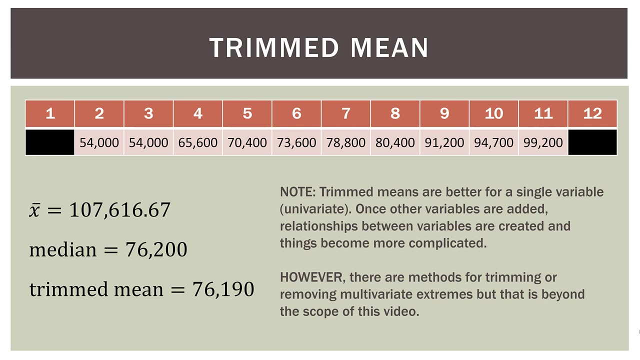 and our original sample mean is heavily influenced by that person who had a $500,000 salary, among 11 other individuals who had salaries around $75,000.. Now here's a note: Trimmed means are better for a single variable, what we call univariate. 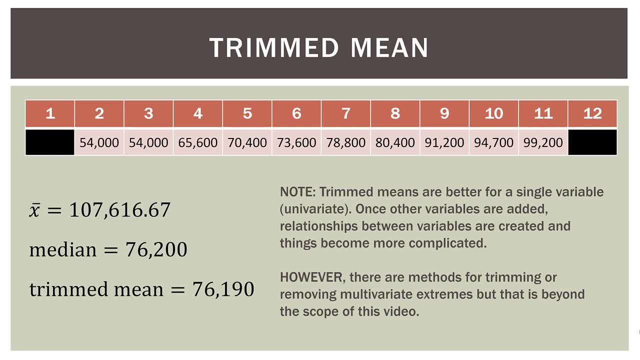 so uni meaning one variate variable. Once you get other variables involved, relationships between variables are created and things become much more complicated. Now, however, there are methods for trimming or removing multivariate extremes, but that is beyond the scope of this video. 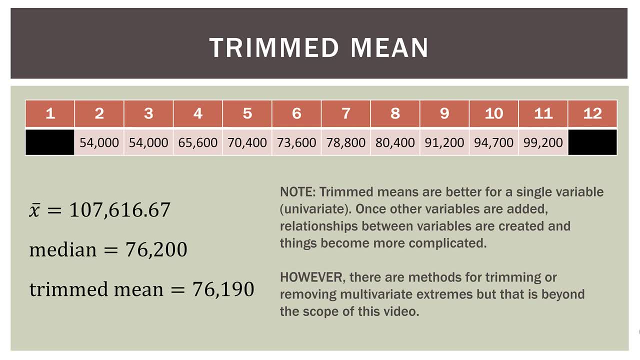 and I do actually talk about that in more advanced videos in my playlists. So when you are doing a univariate analysis, what I would recommend is reporting all three of these values. Report your original sample mean, the median and then a trimmed mean.